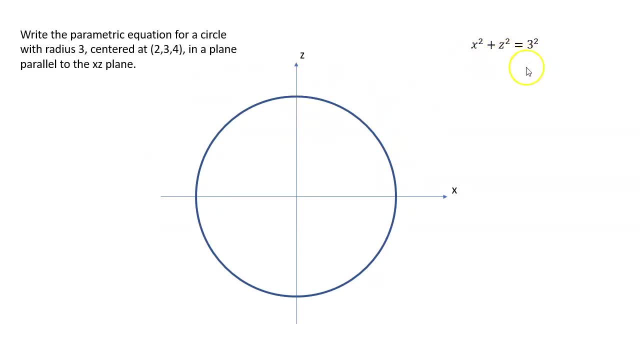 Now normally you might think: oh, I would write the equation as: x squared plus z squared equals radius squared 3 squared right, And that works fine for sort of a standard equation in 2D, but for 3D we're going to need to parameterize this equation. 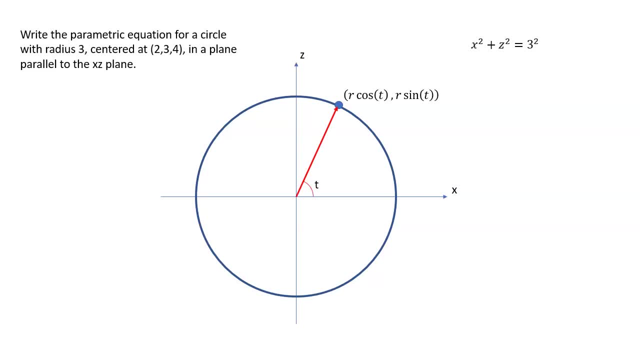 So the way we're going to do that is we're going to take a, we're going to relate it back to our trig knowledge And we're going to treat t as if it was the angle here, And remember that the coordinates of a point on a circle 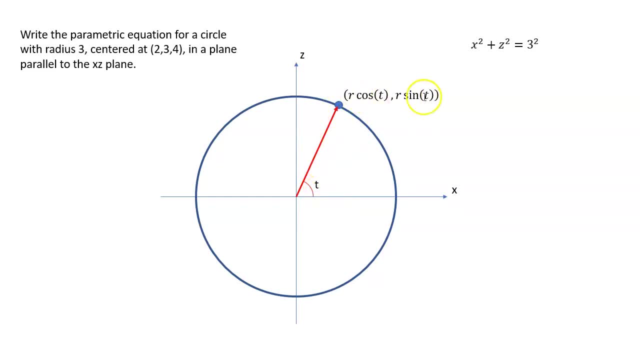 at an angle of t, are r cosine theta and r sine theta. or again, if we're using t as the angle, r cosine t and r sine t, And that lets us create our parameterization: x equals r and our radius here is 3,. 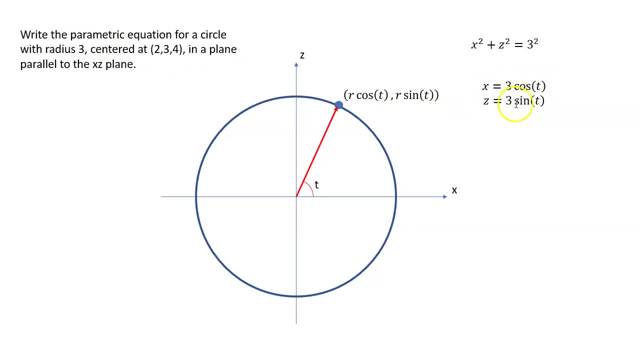 so x is 3 cosine t and y is 3 sine t. So we're going to use a cosine and sine pair to create our rotation, to create our circle. And in case you're wondering how this equation relates to the original equation, 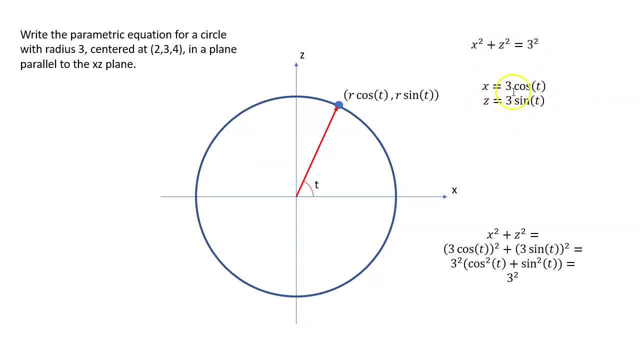 notice, if you were to take x squared plus z squared and plug in these two formulas here, we would end up with a cosine squared plus sine squared, which is 1, and we'd end up with our 3 squared. So this equation, these parametric equations, 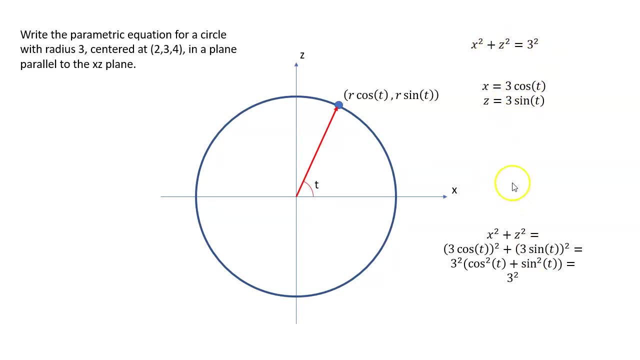 do satisfy. x squared plus z squared equals 3 squared, All right. so in order to parameterize a circle of radius 3, we can use: x equals 3 cosine t, z equals 3 sine t. It's that cosine and sine pair that give us the rotation. 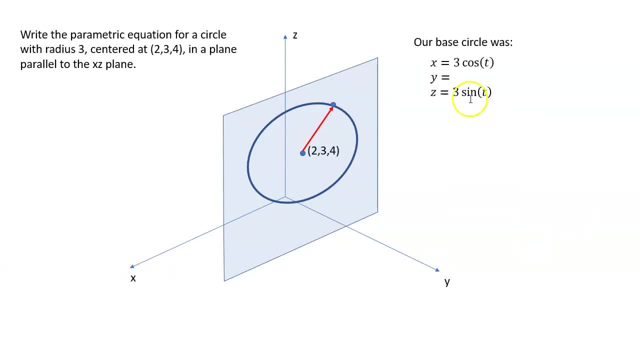 All right, so let's pop back into 3.. Now, right, our base circle had an x of 3 cosine t as z of 3 sine t, and we weren't really concerned about y. But now we need to shift our whole circle up. 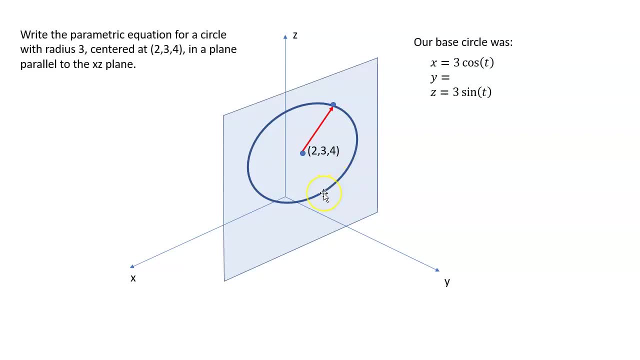 so that the base point is at 2, 3, 4.. And we need our rotation to be happening around 2, 3, 4.. And we really can do that just by taking our equations and shifting them by the amount of the center point.